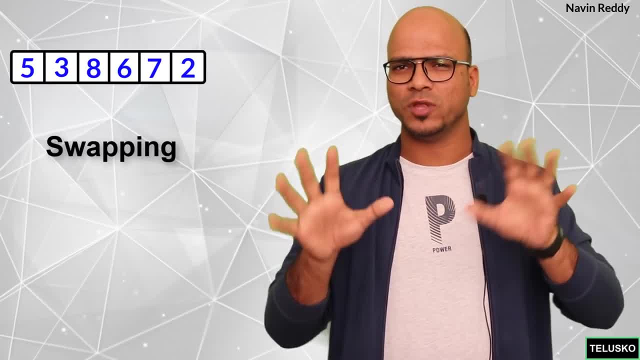 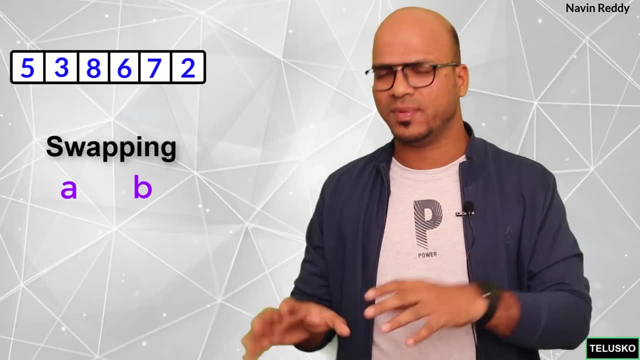 of the important concepts. So make sure that you know the concept of swapping. So what we normally do is we take a third variable here. So, example: if you have A and B and if you want to swap them, You will take a third variable, let's say T, and you will keep the value of A in T. Then 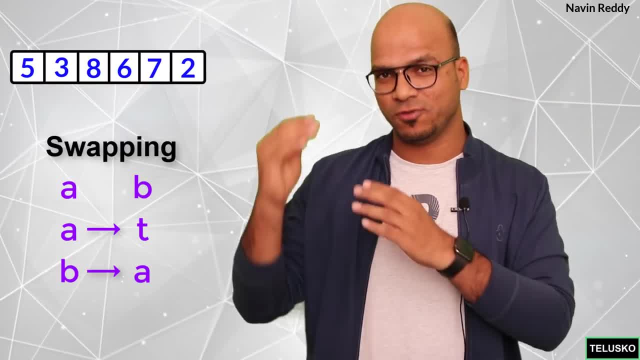 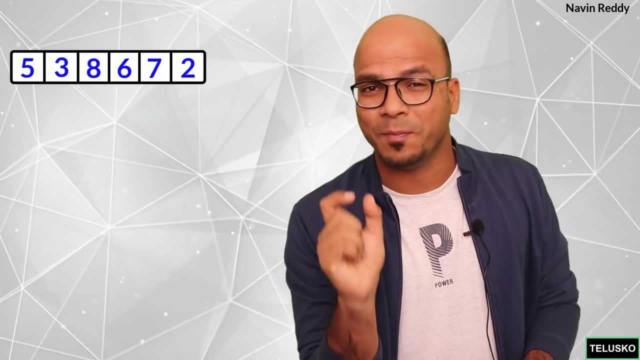 you will copy the value from B to A and then you will copy the value from T to B. That's how you swap two values, And we'll be doing that in this video as well. Let's start with the swapping itself. So what we'll do is we'll compare the first two values, In this case, 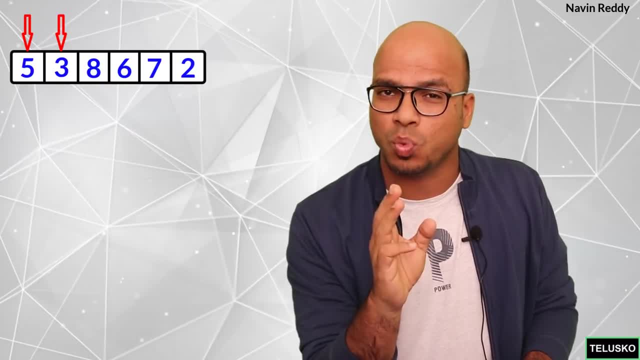 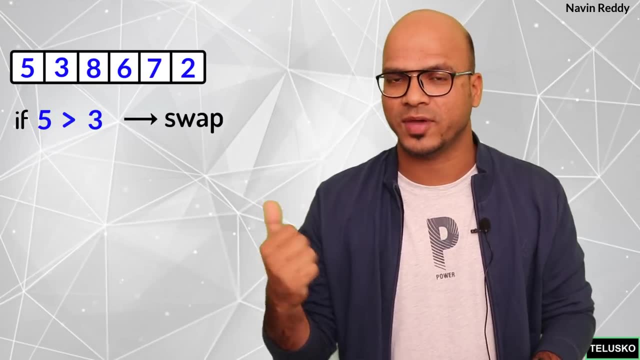 it is 5 and 3 right. Now. you have to make sure that the smallest one comes first, So you will compare if the first value is greater than the second value swap. In this case it is greater, right? So 5 is greater than 3.. 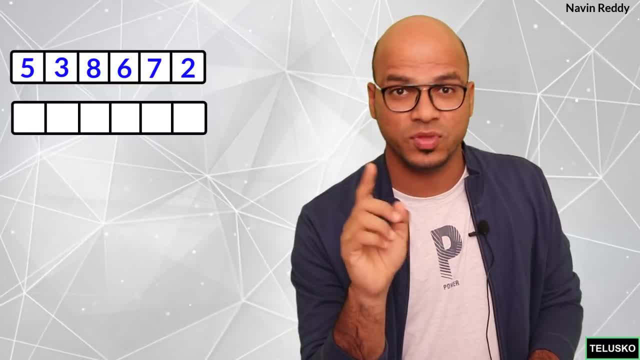 So what you will do? you will swap it. So now, after swapping, the values are 3,, 5,, 8,, 6,, 7,, 2, right, And now what you will do is: now you will iterate, Now you will go forward. 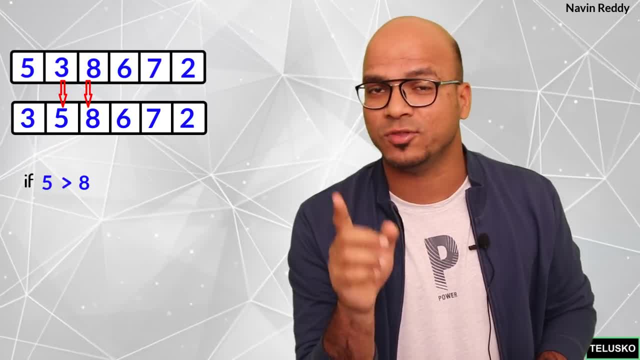 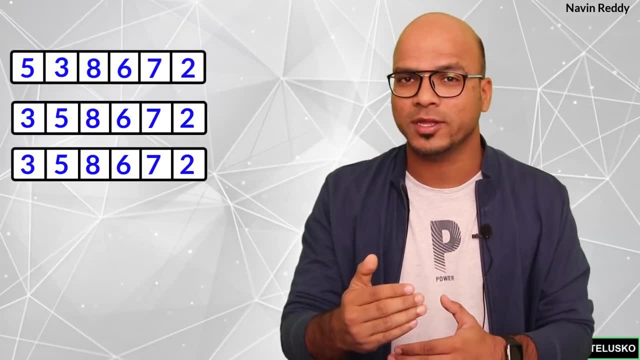 So we have to make sure that if the first value is greater than second value, then swap, otherwise skip right. In this case, it is smaller, right? We don't have to swap now. Now, what you will do is you will iterate. At this point, you will compare 8 and 6 right Now in this. 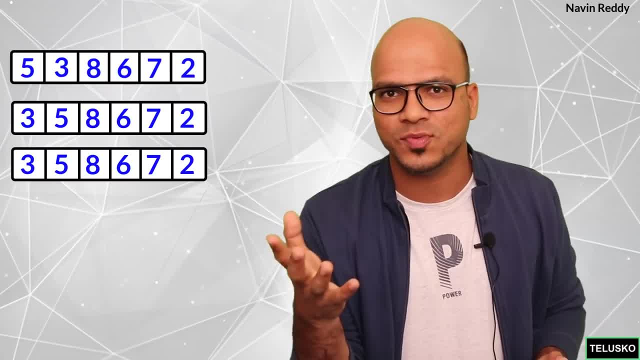 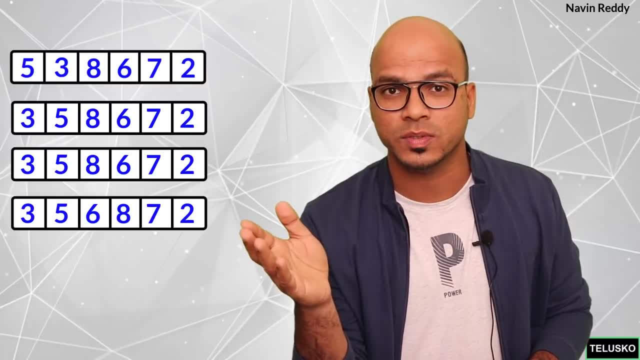 case 8 is greater than 6. right Now, you have to swap as usual. right Now, after swapping, you will get 6 and 8.. So the final value you will get is 3, 5, 6, 8, 7, 2.. Okay, that's great. Now you have. 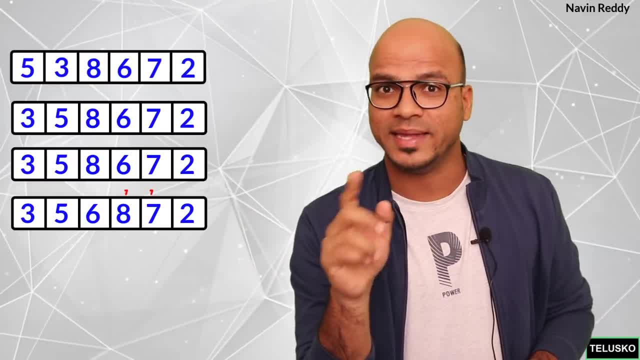 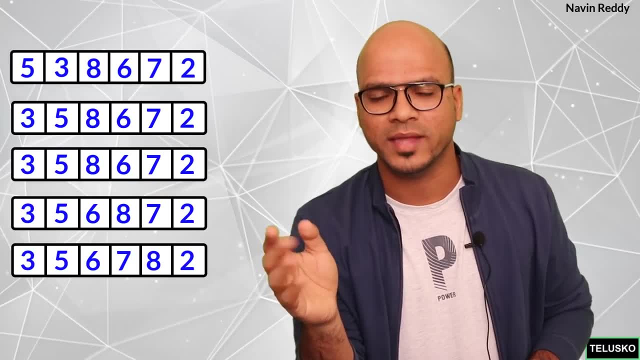 to do the same thing till the end. So let's make it quick. So now you will compare 8 and 7, right? Again, we know 8 is greater than 7, so we will swap. The new value you will get is 3, 5,, 6,, 7,, 8, 2, right. And the last comparison: we have 8 and 2, and of course we know we have. 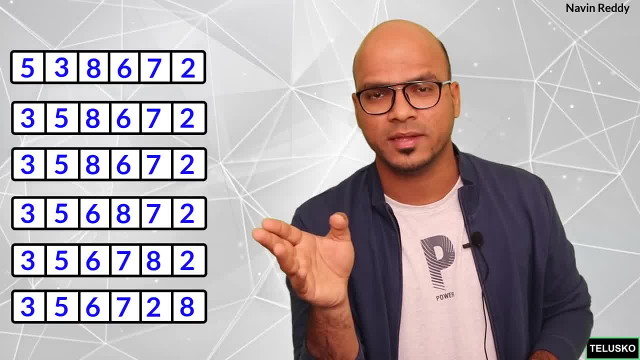 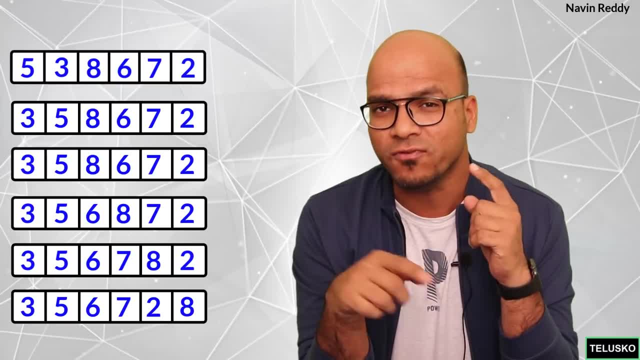 to swap. So at the end, you will get 3,, 5,, 6,, 7,, 2, 8.. Now, after this iteration, after doing all these things, we have got one thing which is 8 at the end. So this is the first iteration, okay, So after doing all these things, you got the biggest. 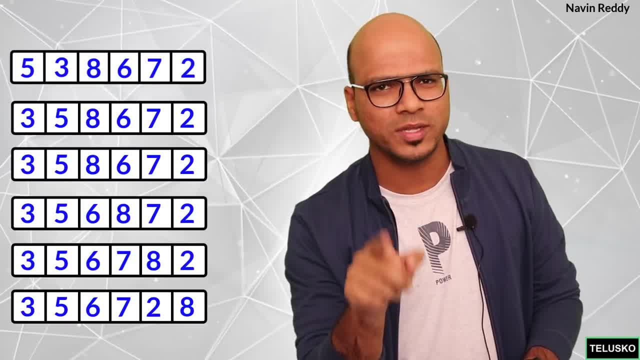 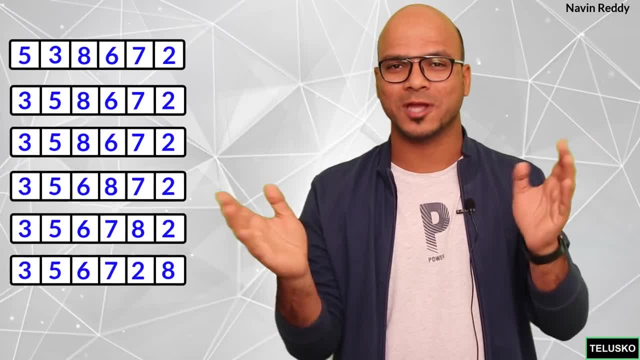 value at the end, But then the remaining values are not sorted right, And now we have to reiterate the same thing. So we have to do the same thing again, And that's how bubble sort works. It's all about comparing and swapping. Now you will start again. Now you will say again: 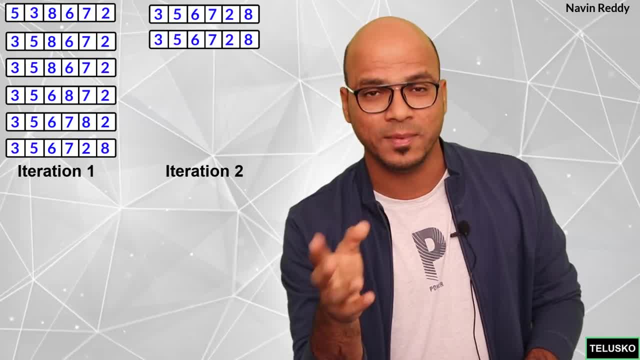 you will compare the first two values, which is 3 and 5.. 3 is smaller, don't have to swap. Then you will compare 5 and 6.. No need to swap. Then you will compare 6 and 7.. No need. 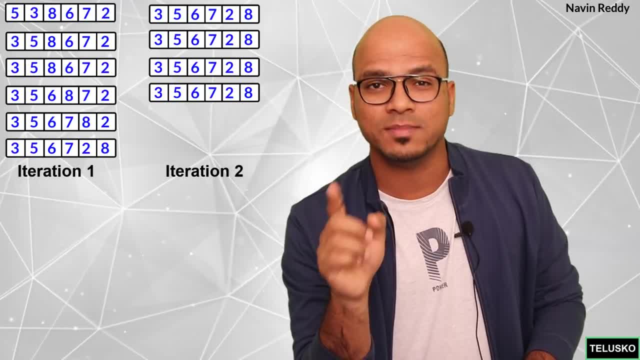 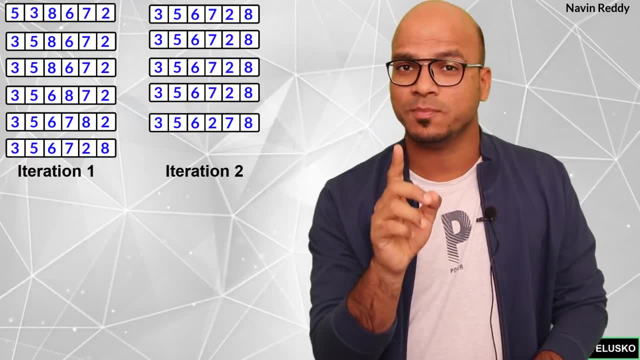 to swap, Then you will compare 7 and 2.. Oh, we have to swap here. Then it becomes 2 and 7, right? So the final values are 3,, 5, 6, 2, 7, 8.. There is one thing which is important. 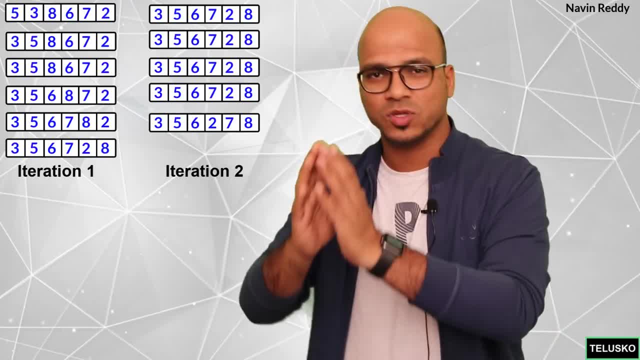 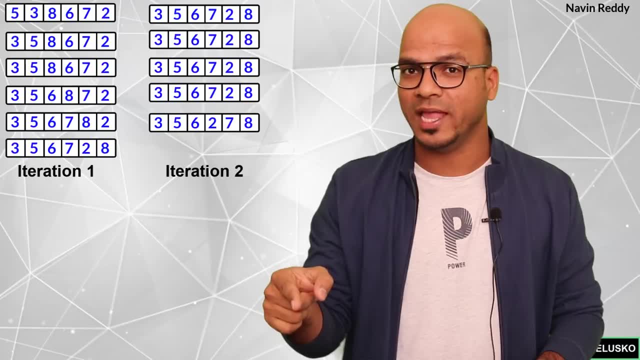 For the second iteration. we are not checking for 8 right because 8 is done. So the maximum value you have is at the end right And after second iteration. the second last value is the second big element. If you can compare the list now, 7 and 8, those are the maximum. 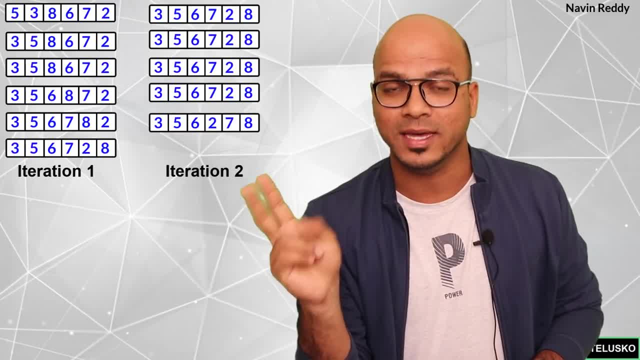 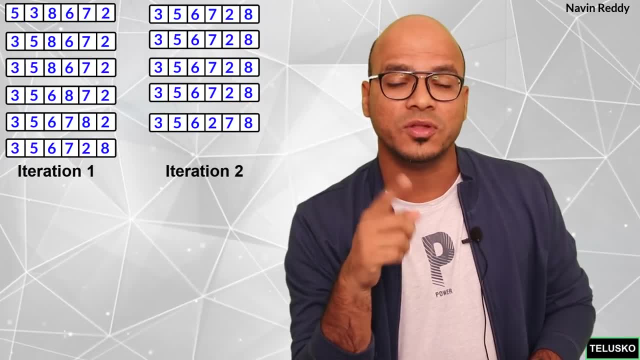 value. So after second iteration you got two big values in ascending order, right? That means after all the iterations. So number of elements we have We have here is 6 right? So after fifth iteration you will get all the values sorted right. 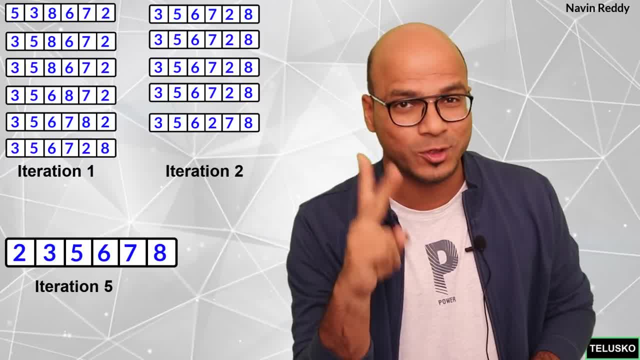 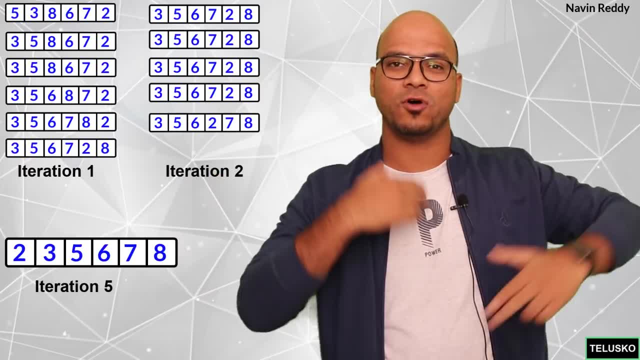 If you repeat the same step. That's what bubble sort is, and that's why we require two loops: One for the iteration, which will make sure that you will get the biggest element at the end, and the second loop, which is the outer loop, will be for do the same thing repeatedly. 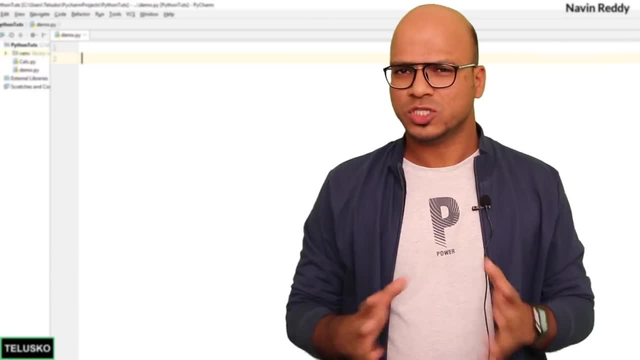 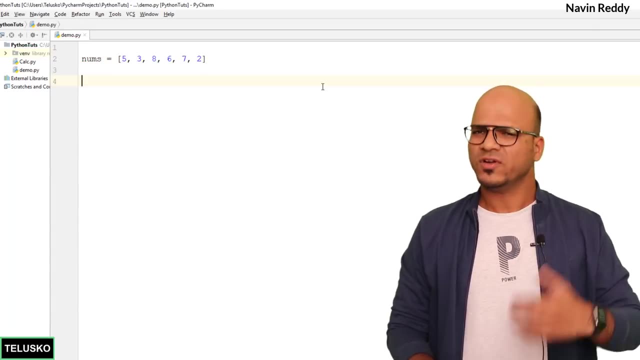 And that's what you have to do in this code. So let's get started with the code here. So it's quite simple. What you will do is you will take a list. So let me take a number list and let's assign the same values we had. 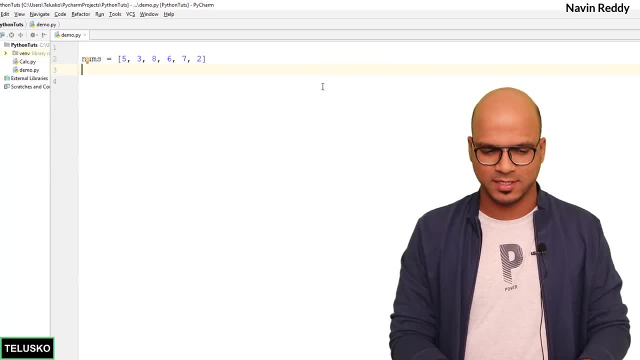 Now, once you've got this value, You will simply say, hey, I want to sort these elements. Now, the amazing thing is we do have inbuilt sorting techniques, right, But then we'll not be using that, we'll be implementing ourselves. So let's say I'm saying, hey, sort, sort this nums here. Now, after sorting you, 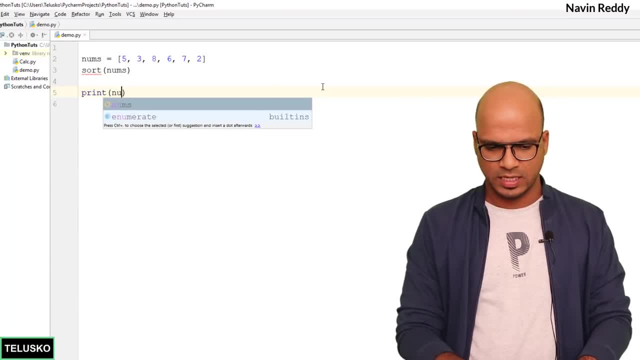 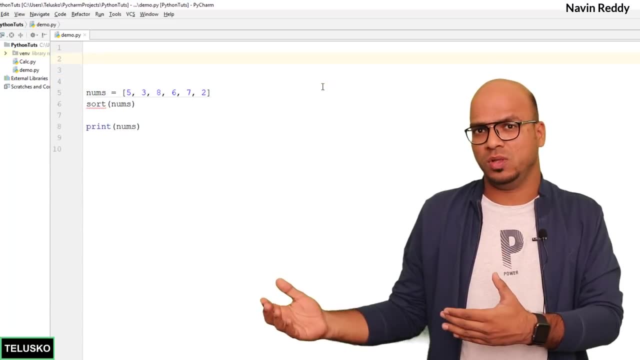 will simply print the values, right? So you will say: print the nums. Will it work? Of course not, right, We have not defined it. So normally you can define this sort method in some other module, or you can do that here itself. Let's do it here. So you will say: 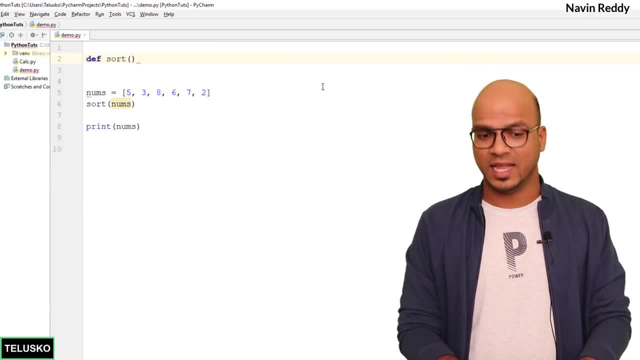 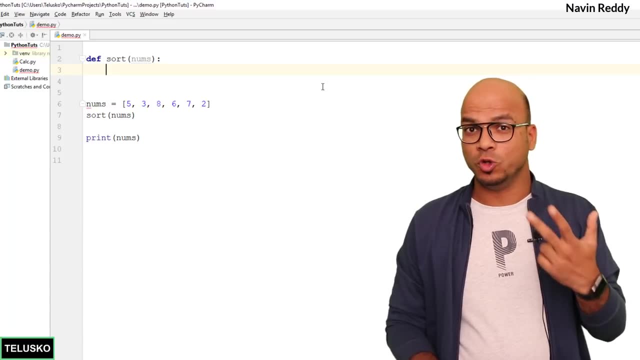 def, And here you will do the actual magic. See, at the end it's all about swapping, right. So you have to take two loops. So we'll take a loop here. So you will say for and you will use I. Normally we can use any variable name, but then I makes sense for the outer loop. 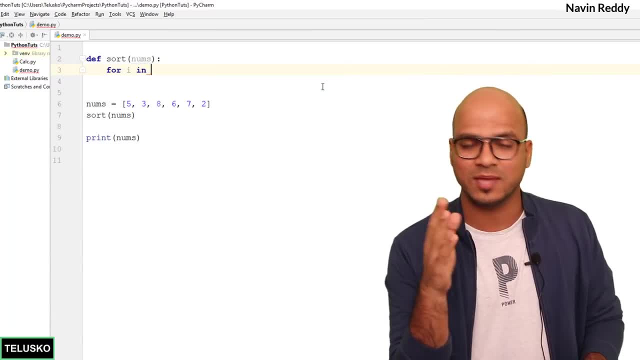 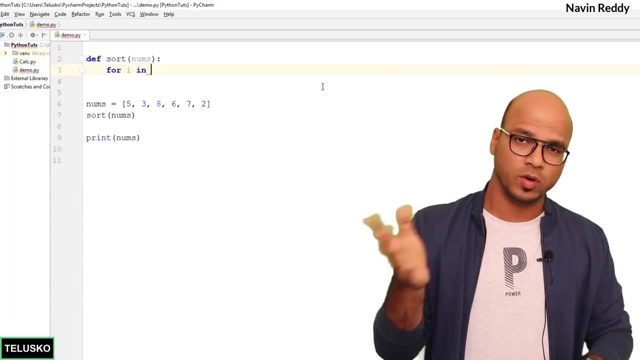 Let's say, for I in Now. the first question is how many times you have to do this, And the second question is in which way we have to do this. Maybe you can do it in descending order. You can do it in ascending order. What we'll do is we'll go in a range, So we'll 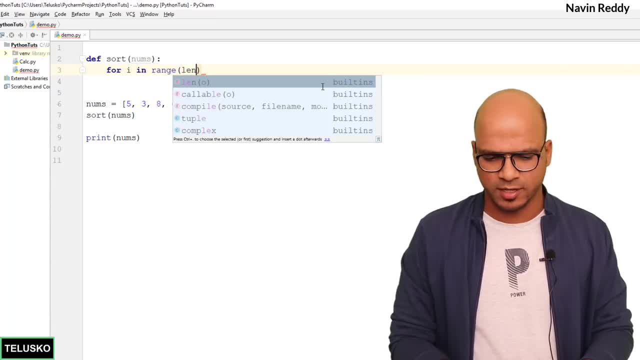 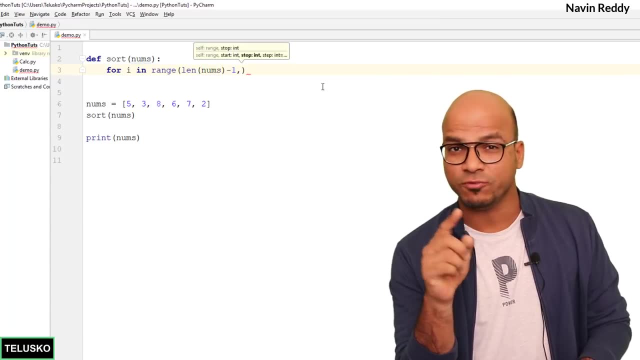 use a range here, But then from when the range will start? I want to start the length of the nums, right, So you will say length of the nums. The idea is, your index number starts with zero, right, So we'll say minus one, And then we have to reach till zero. So we are going from. let's. 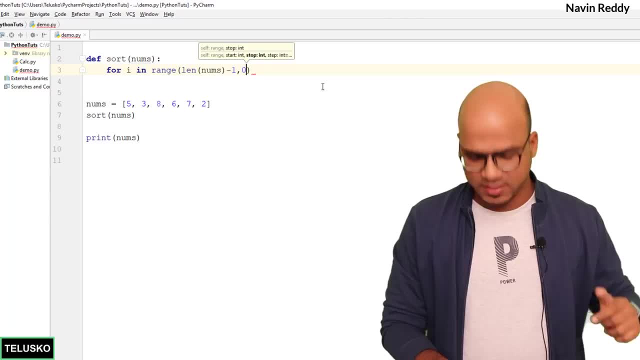 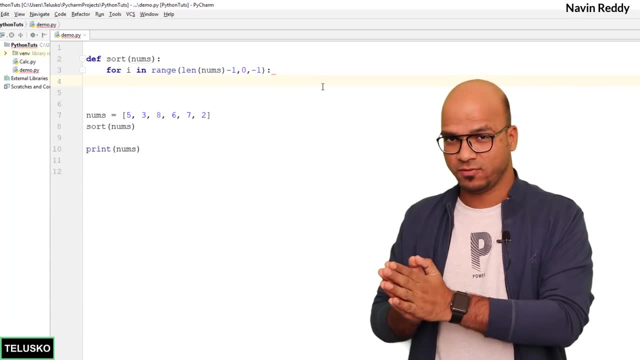 say the length is six, We are going from five to zero, And since we are going in negative order, so we'll say minus one, So the iteration would be minus one here. That's how we use range, right? So basically we're going from five to one. Now, once you've got the outer, 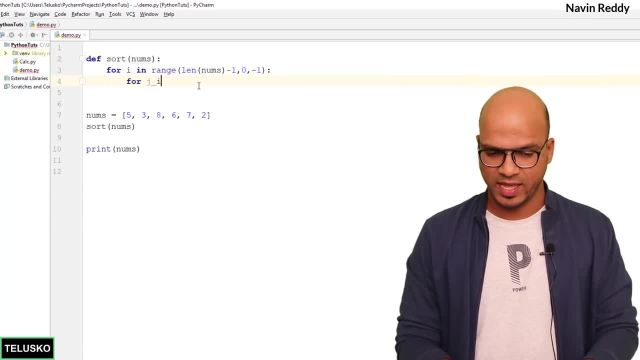 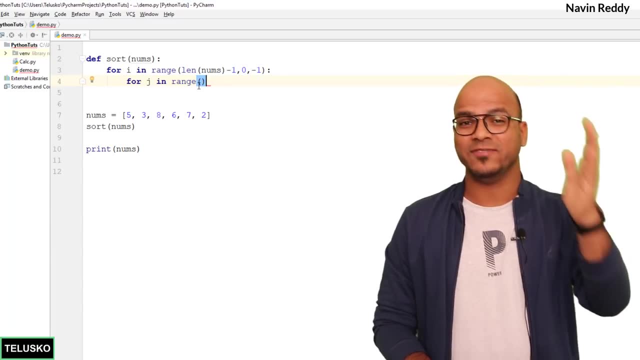 loop. now it's time to go for the inner loop. So we'll say for j in. Now we have a different range here. So for the first iteration, if you remember, we have to go till n. right, We have to start with zero and we have to reach till five. In the next iteration, we have to 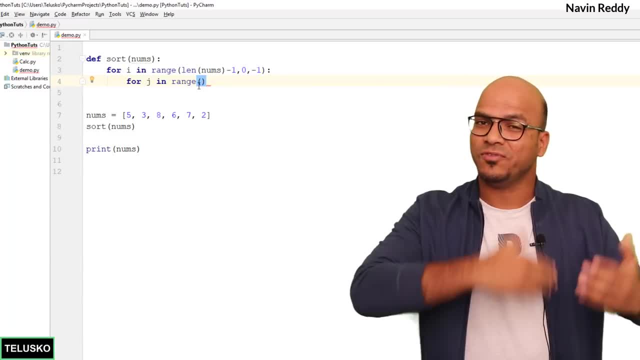 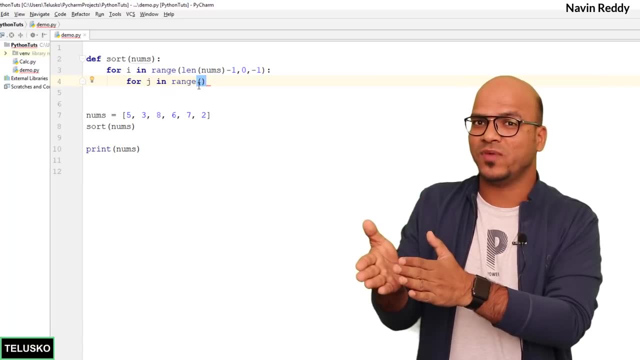 go from zero to four In the next iteration. we have to go from zero to three. After every internal iteration you will get the maximum value at the end. Then second last value will be the second biggest value. Third last value will be the third biggest value, And that's. 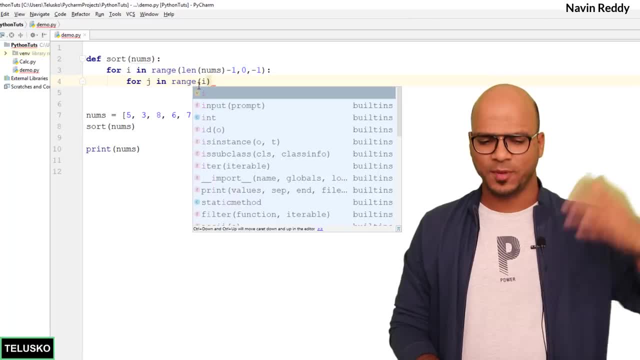 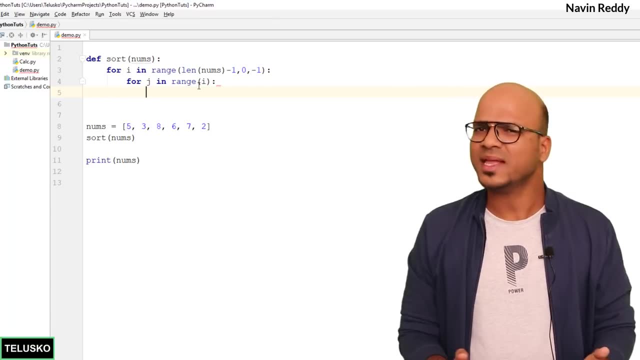 why the range will go till i, not five. It will go till i. So they've given up on the value of i, which is five. It will be five. If it is four, then it will be four, Because after every iteration we are getting one value fixed And that's it. So that's how we do. 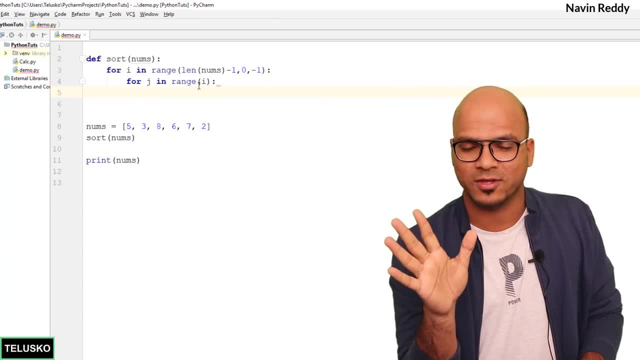 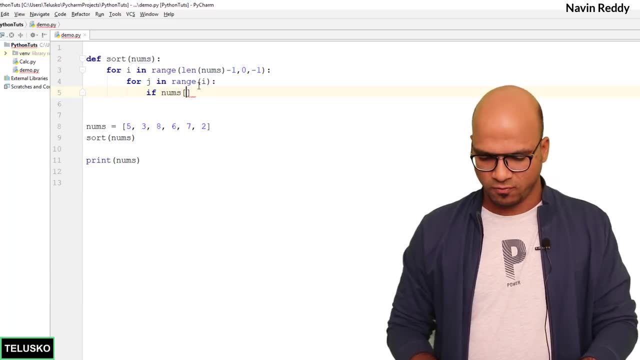 it. That's it. This is your loops. Now we just have to decide one thing: Should we swap the values or there's no need to swap the values? That's it. That's how a bubble sort works, So we'll simply check. If nums of j is greater than nums of j plus one, then we have to swap. 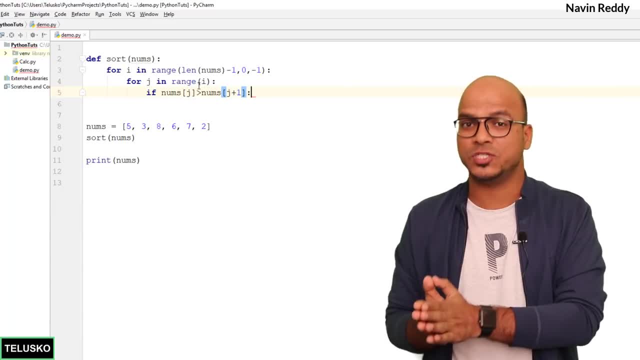 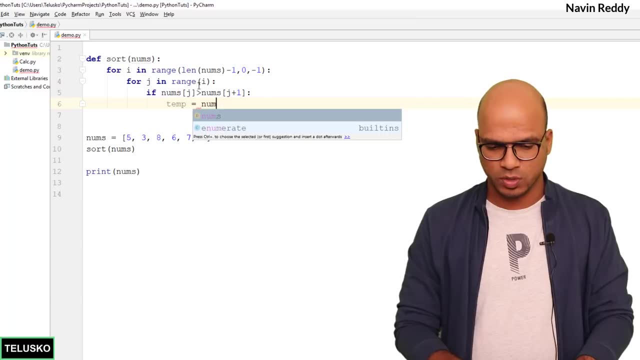 right, That's what we did in theory, right? So if the first value is greater than second, value swap. How do we swap it here? It's very simple: You simply use a temp variable. Temp is equal to nums of j, And then you will say nums of j is equal to. 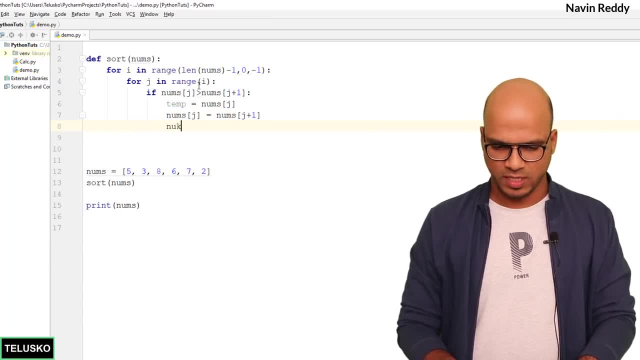 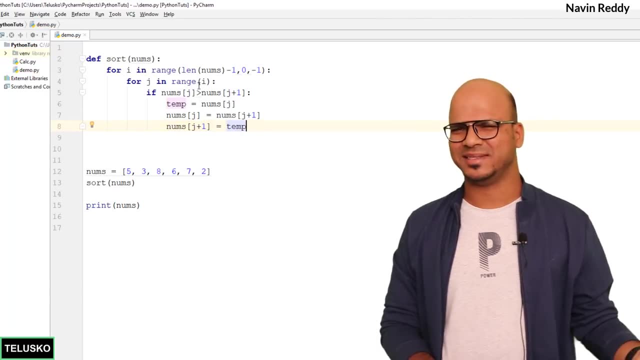 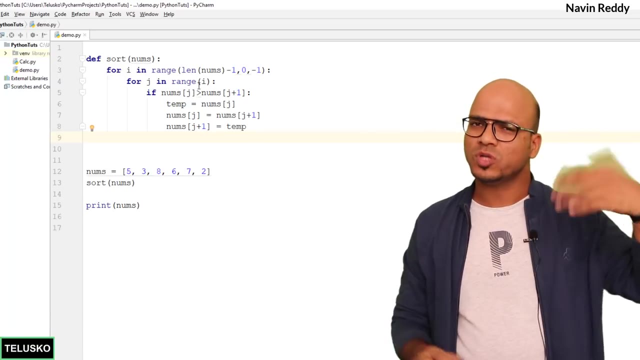 Nums of j plus one, And you will say: nums of j plus one is equal to temp. That's it. That's what you do. We need to make sure that you use two loops, One for the external, one for the internal right. So the internal loop will do the swapping. The outer loop is just.